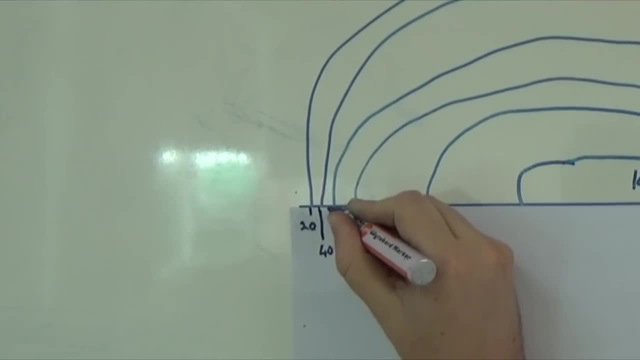 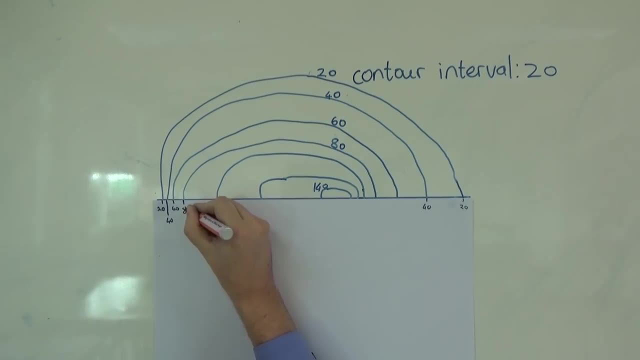 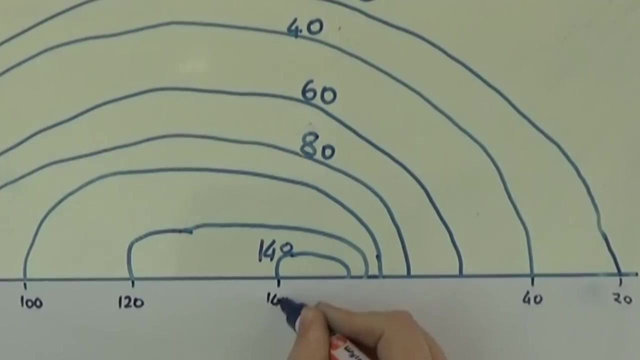 line down, And then the next one we know is 60. Then we go to 80, 100, 120. And then, as we can see, this line here is 140.. This is once again going to be 140.. Now, 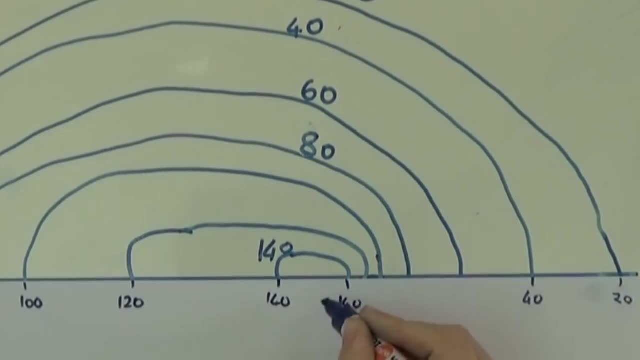 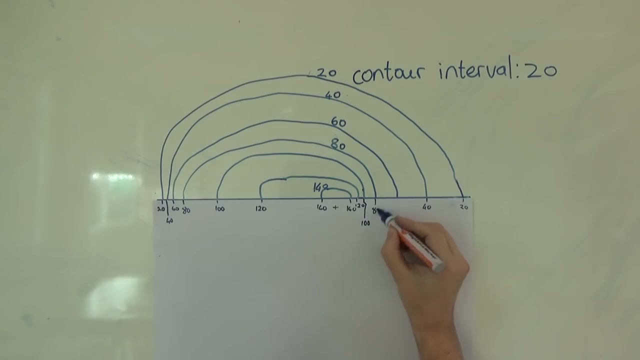 here is where you must make a note to remind yourself that this area here between these two lines, or where these lines cross the horizontal line, is higher than 140, unless there's something strange going on there. But so make a plus here. Very important to place your piece of paper. 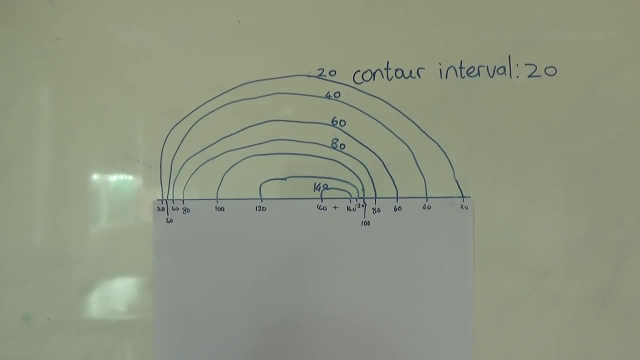 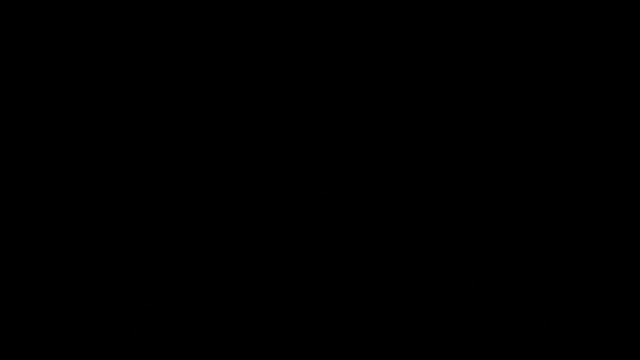 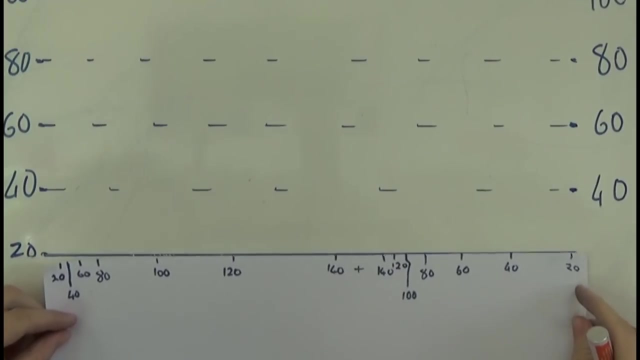 properly and make sure it doesn't move, Otherwise your cross section won't be accurate. Right, let's go to step number two. Okay, step number two. Now, once again, it's very important not to let your paper slip. 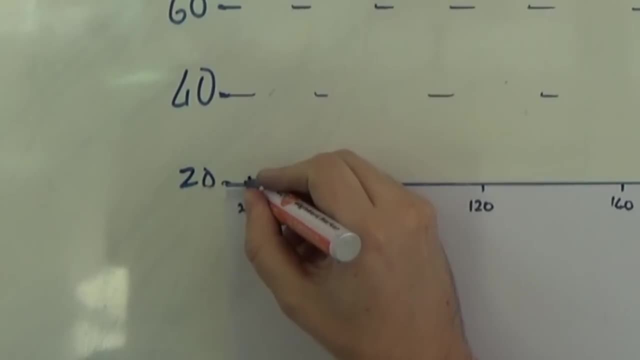 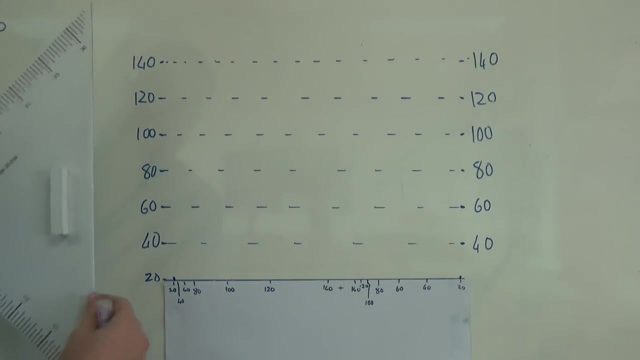 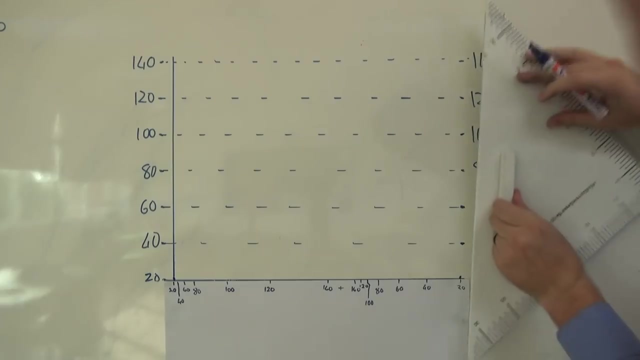 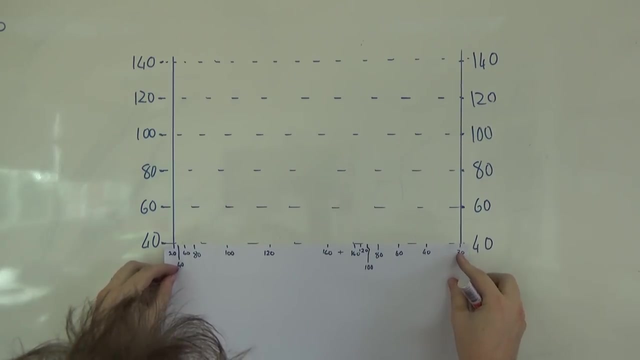 And here we have 20.. So you just make a little marker there. Same on the other side. I just want to make 100% sure that I'm working accurately. Now we are going to move them up. Make sure that you line up your piece of paper as accurate as possible, And here is where we are going to make. 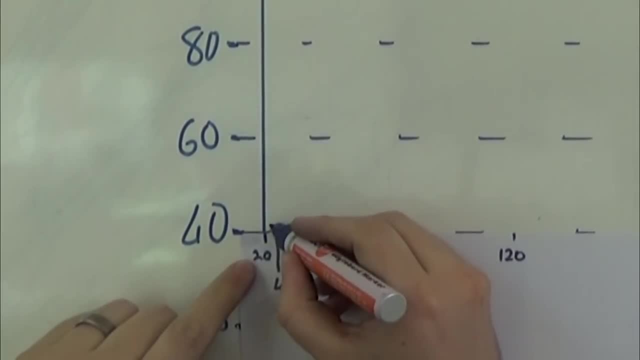 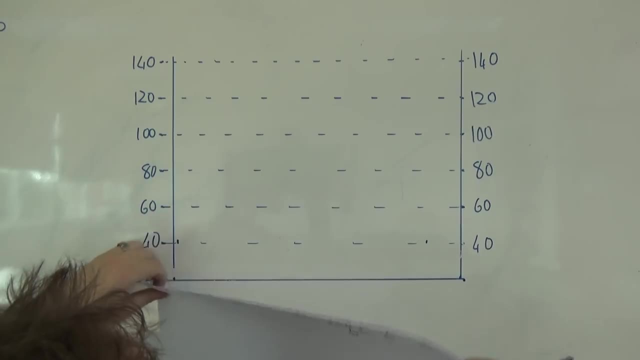 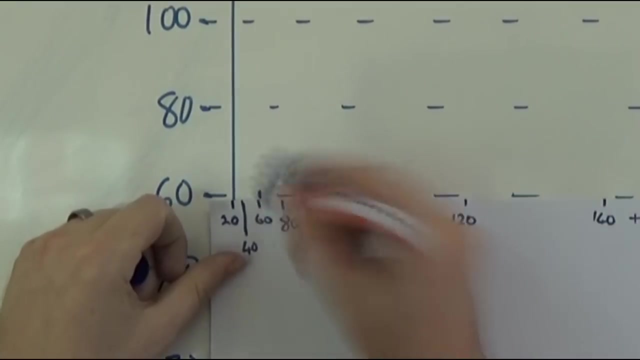 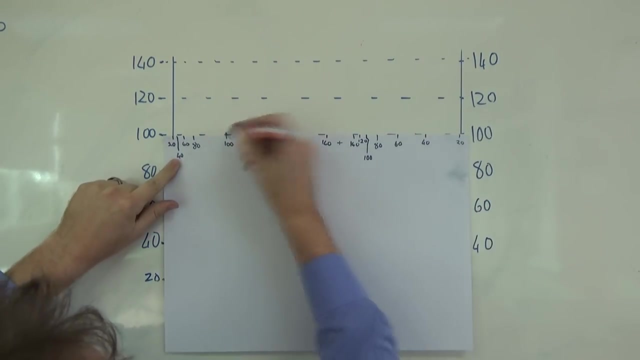 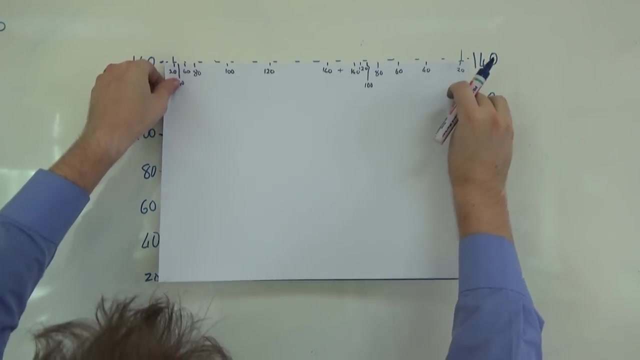 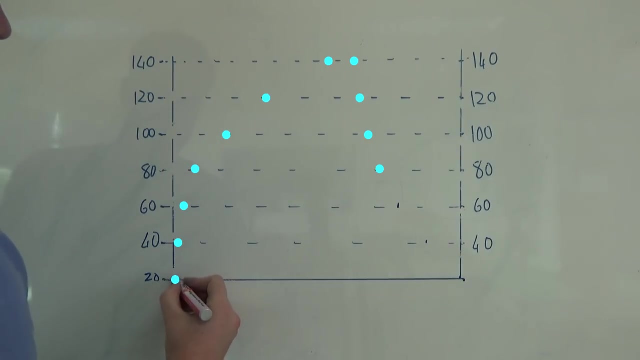 the next marker There we can see this is 40.. 40 is over there, And then we move the paper up once more up to 60. So now we are going to connect these markers. Here is 20.. This is a very steep slope, as you can see.